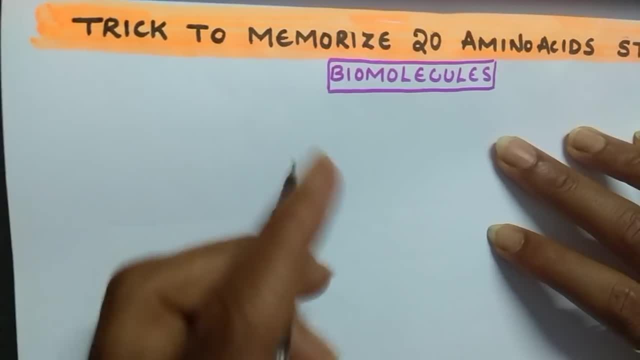 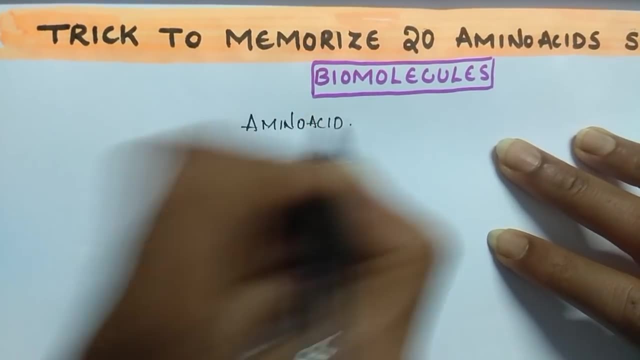 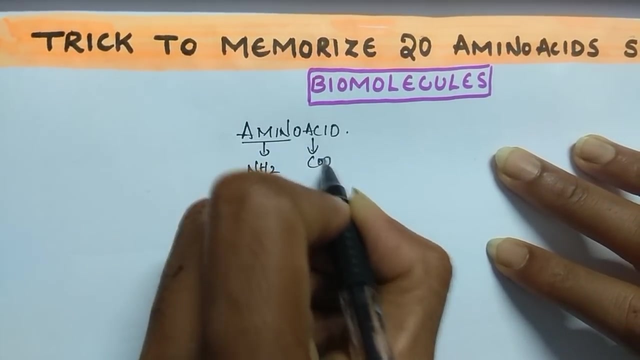 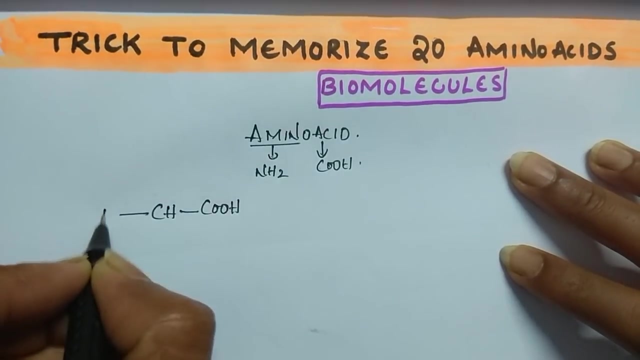 in this video. Let's start the session. Amino acid name itself: it is clear that amino amino acid name itself. it is clear that one amino group will be there, Amino group and an acid group. So general structure is CH, COOH. it is having and it is. 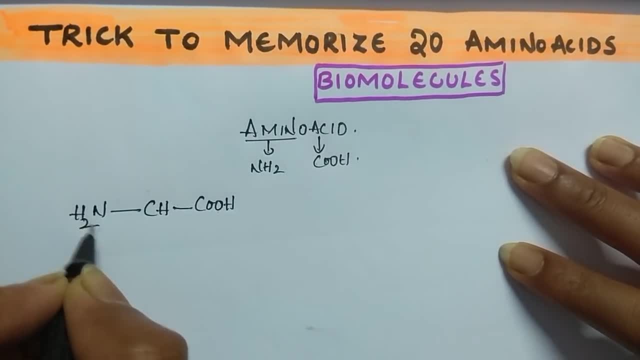 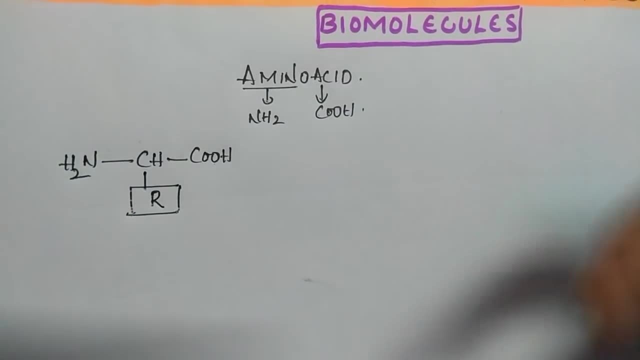 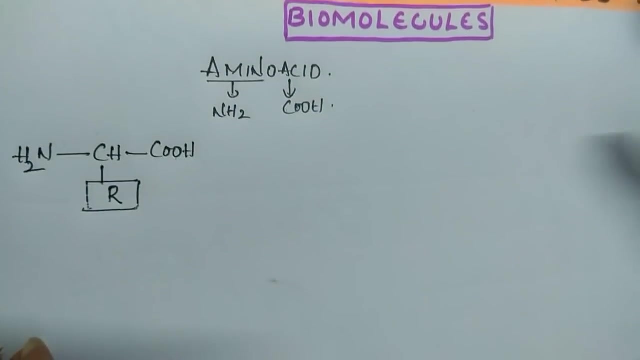 having one amino group, an acid group and an amino group and an side chain. This side chain varies. This R place we keep different alkyl groups and based on that, we are going to get different structures of these amino acids. Clear and this is a structure. 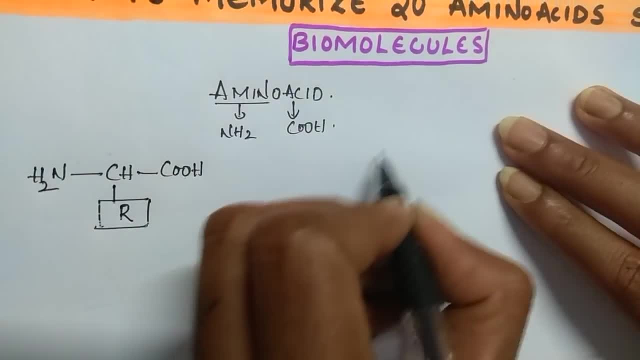 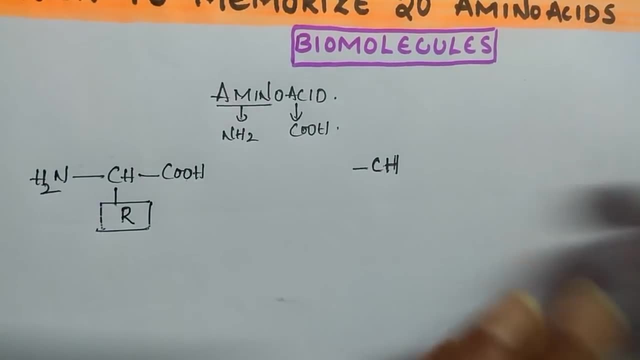 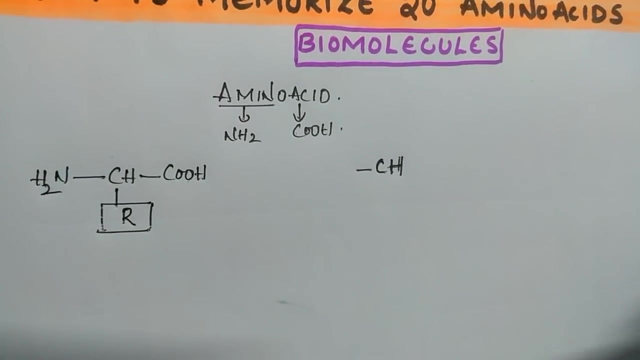 Same structure. I am going to write in ionic form. What is this ionic form? See here CH. follow the video up to the end and don't copy anything. now, By watching the watch complete video again, take paper and pen and then you draw the structures along with me. Here, NH2 ionic form. I am writing 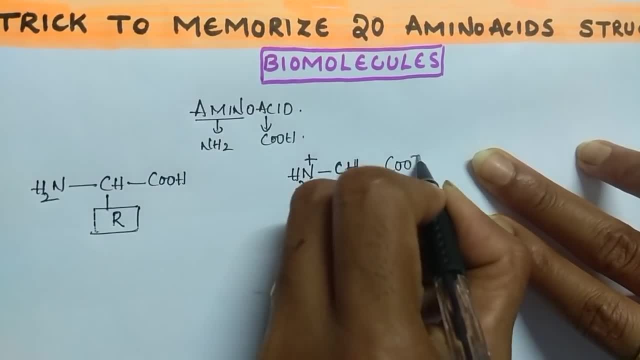 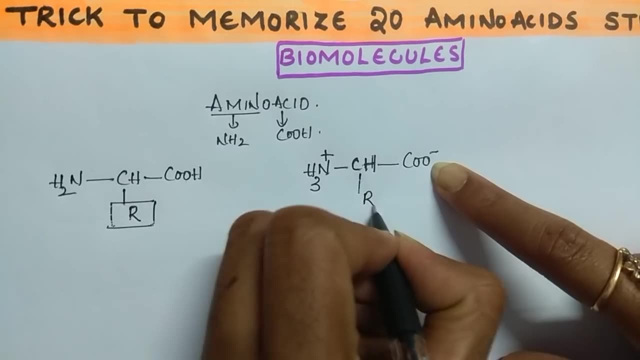 NH3 plus and COOH- ionic form- CO minus. I am removed one H plus from here, So I am going to here and I added one H plus here, Then I am keeping it. This is an ionic form of the amino acid. 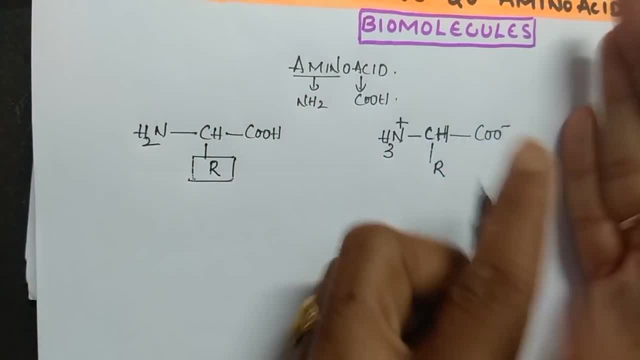 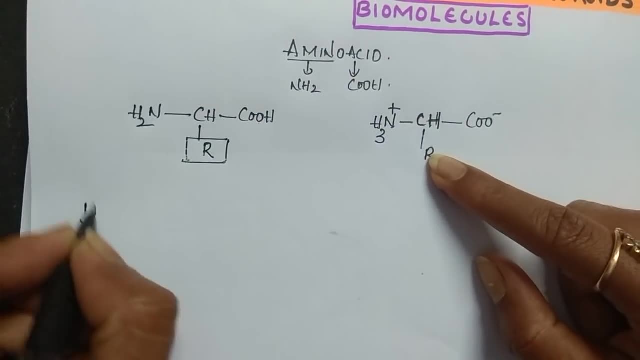 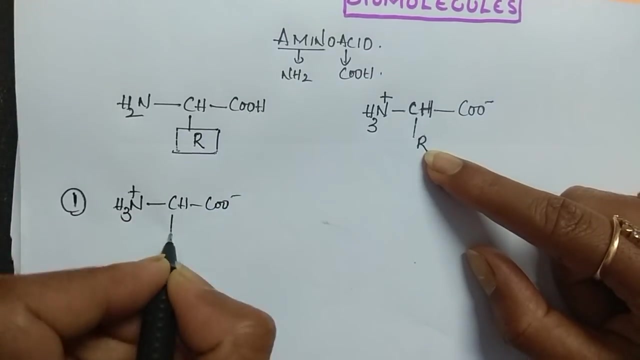 I am going to change this R part. I am using this structure ionic form. You can use this format also. I am using this ionic form. See the first structure: NH3 plus CH, COO minus R place I am keeping hydrogen. Then it's name is glycine. 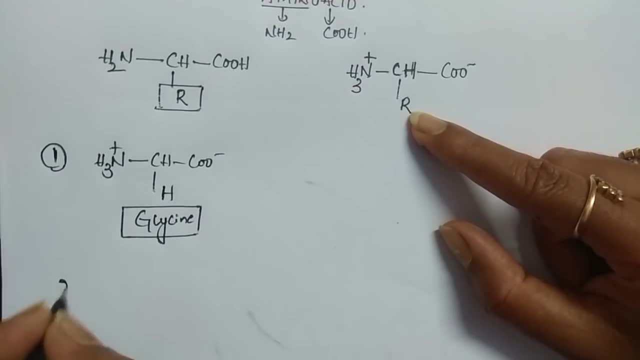 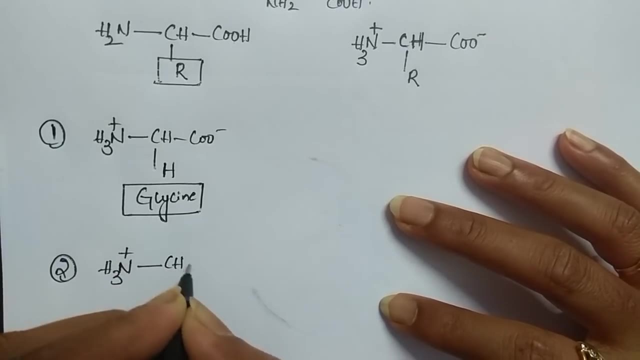 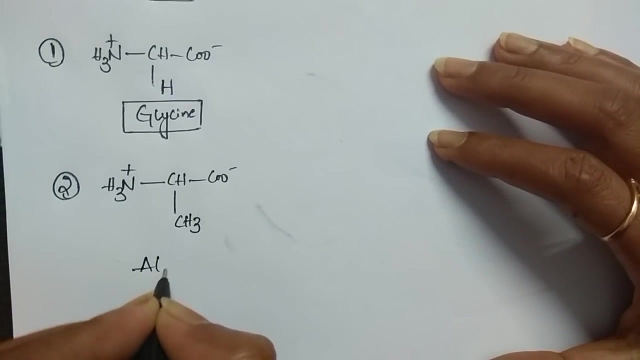 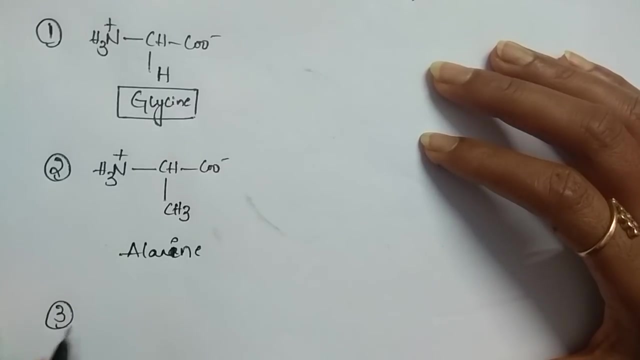 What is the name, students? Glycine, What I kept R place, hydrogen: Same structure, NH3 plus CHCO minus no change, Hydrogen place I am keeping CH3.. Then its name is alanine. What is the name of amino acid? ALA? NINE? Okay, alanine, Third structure: Same structure of this alanine. and what I am going. 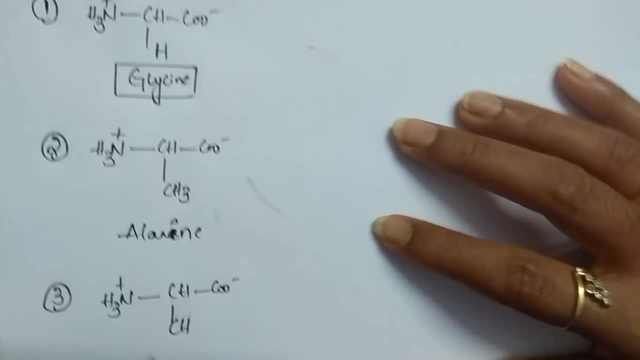 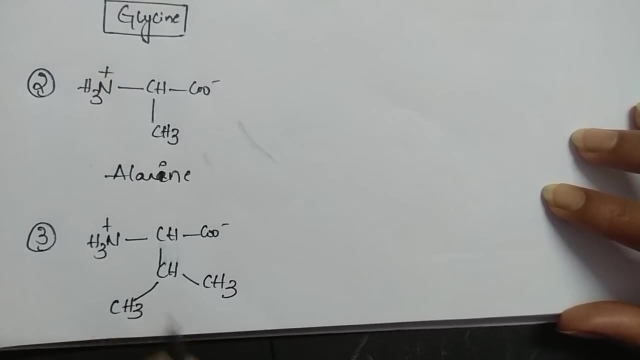 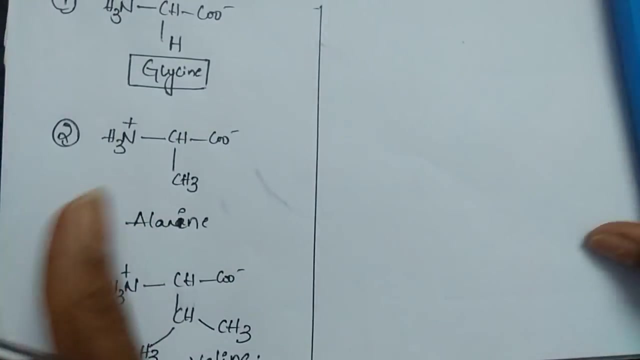 to do is remove two hydrogens from CH3.. One hydrogen place I am keeping CH3.. Another hydrogen place, I am keeping another, CH3.. Valine- Valine- What is the name? Valine. Got the clarity And see the next structure. 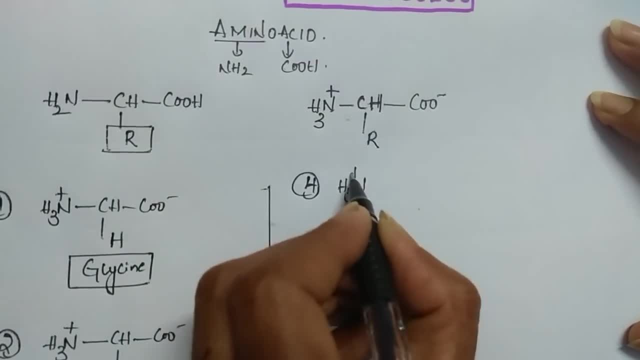 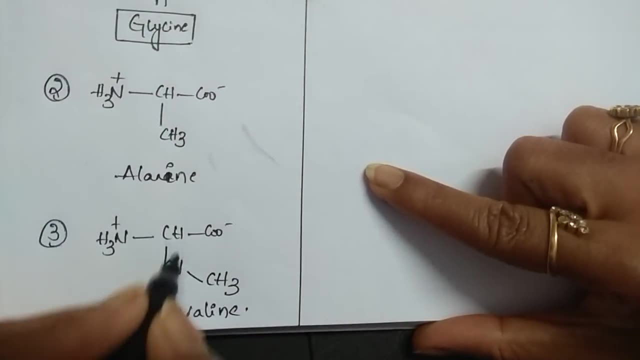 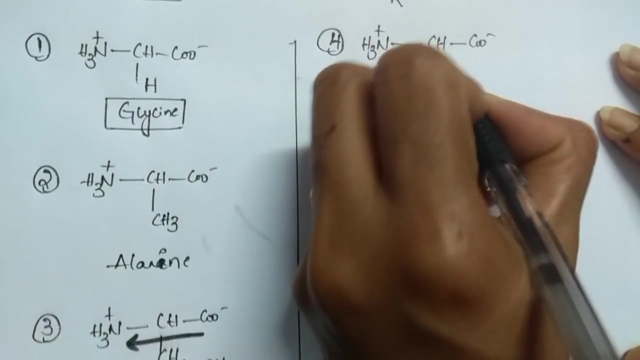 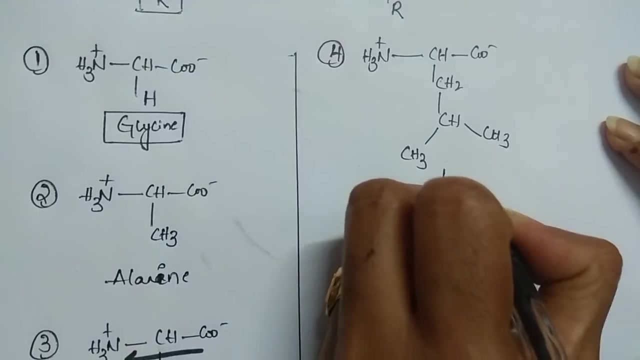 Fourth, one Same structure. I am going to draw Valine structure, But here the thing is: see here same valine structure. Simple trick is: between these two carbons put CH2.. One extra, CH2.. CH2, then CH, CH3,, CH3. This is called leucine, Leucine, Okay, See the next amino acid. Same. 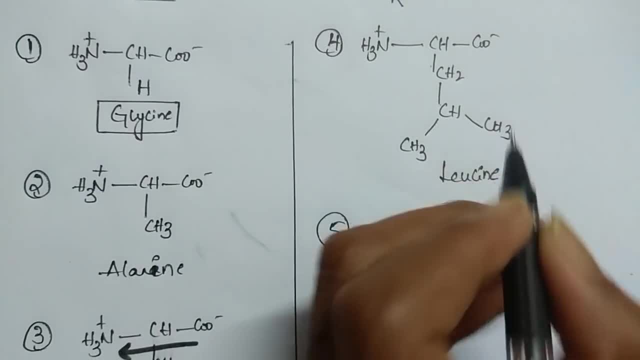 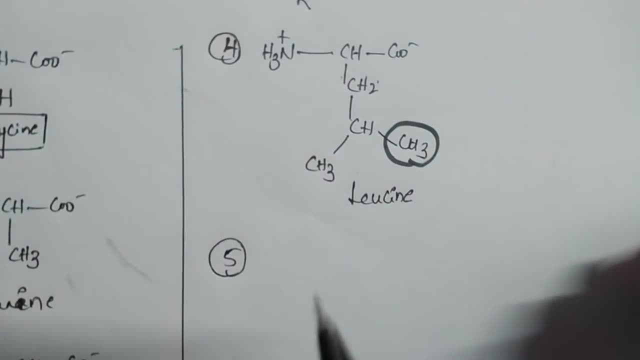 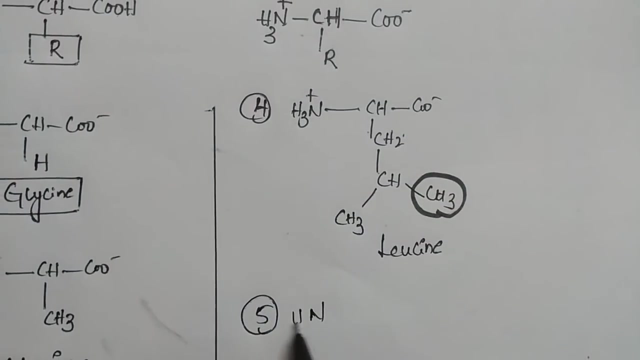 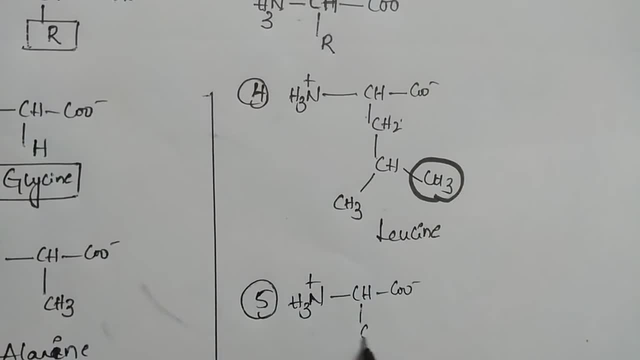 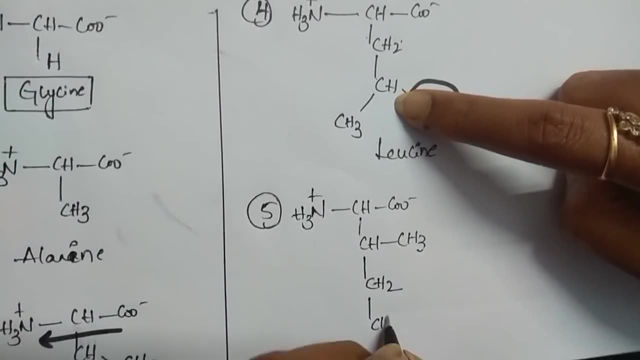 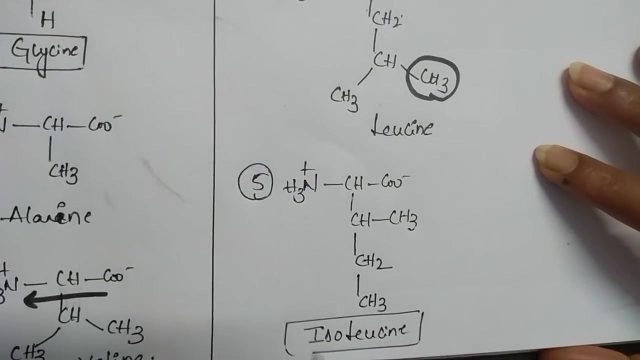 and CHCO minus. and here, just I am keeping CH3.. This CH3, I moved here, and that hydrogen I move here. Then we get a structure. This is called isoleucine Five structure. These five structures are of similar kind. Okay, Glycine. 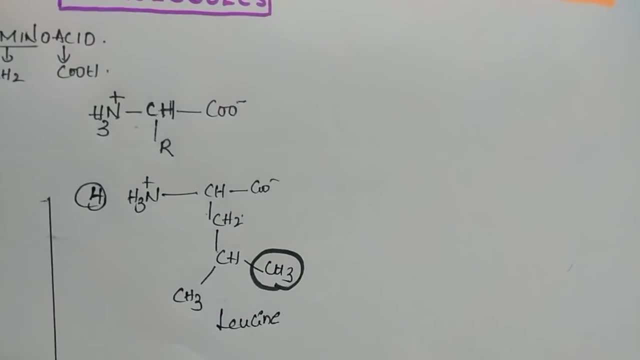 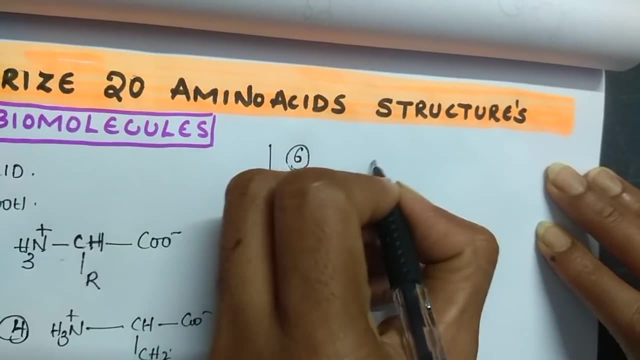 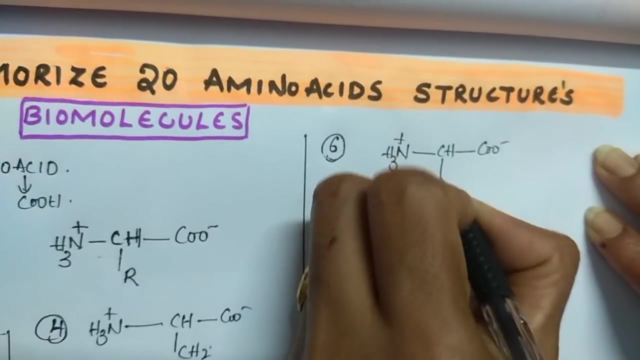 alanine, valine, leucine, isoleucine, Clear, Now I am going to teach you a sixth structure of amino acid, That is, I am going to take same amino acid as alanine, and alanine means here CH3.. Okay, And I? 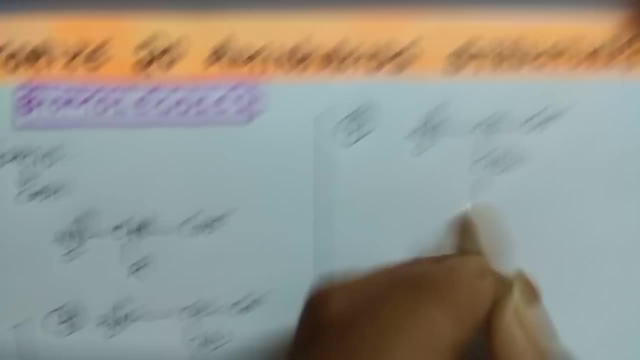 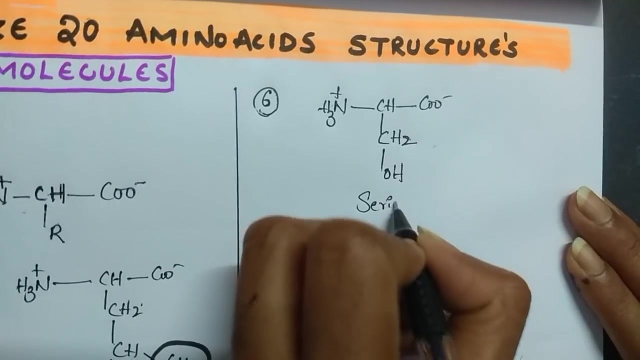 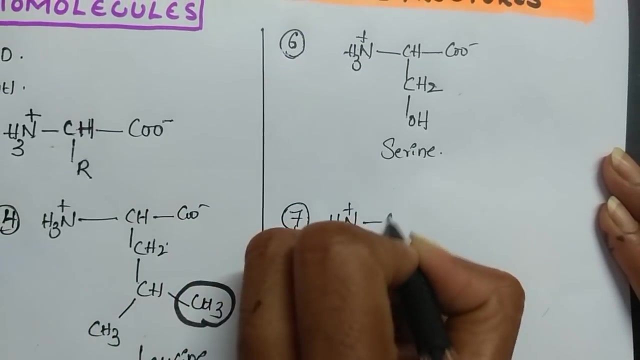 am keeping CH2.. I removed one hydrogen from this alanine structure and I am keeping OH here. Its name is serine Serine. Okay, Next seventh structure. I am drawing NH3 plus and CHCO minus. No change Here. CHOH is: 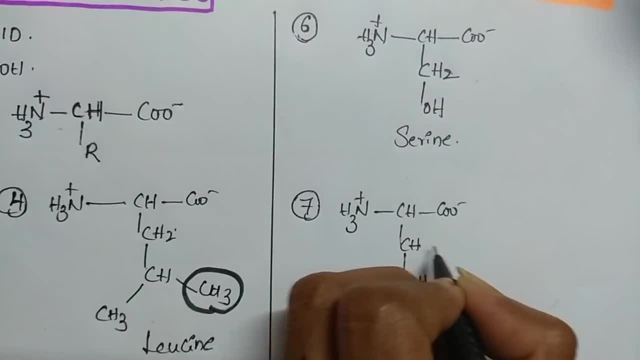 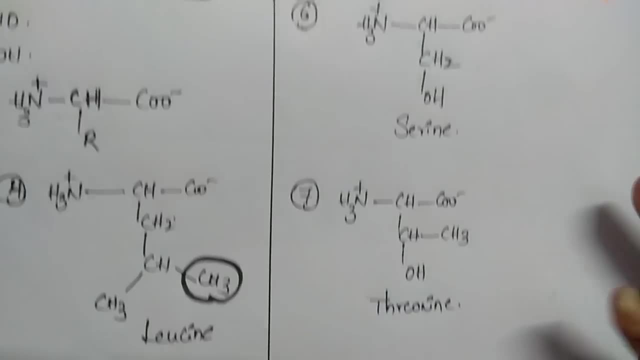 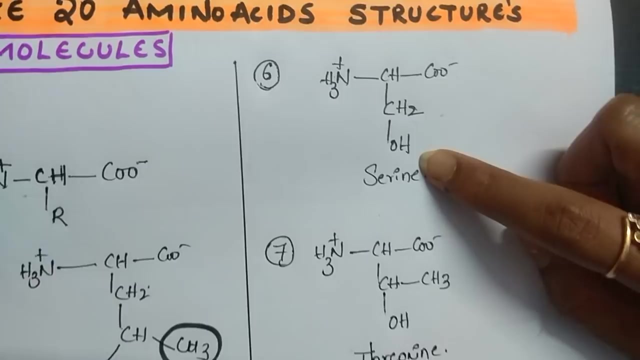 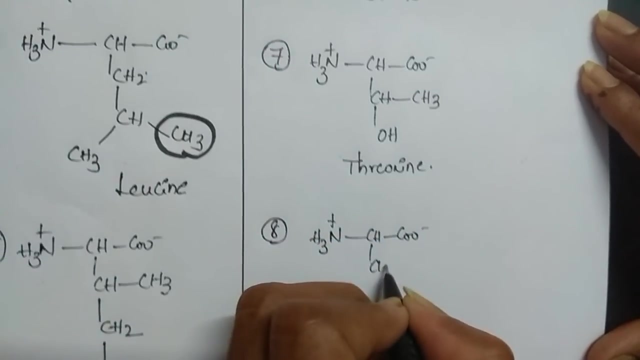 common One, hydrogen from serine. I removed and I kept one, CH3.. Threonine- Easy right Threonine And next structure is: Next structure is Same serine structure. I am taking Same serine structure. I am taking This OH part. I am replacing with OH part. I am replacing with SH. See here SH. 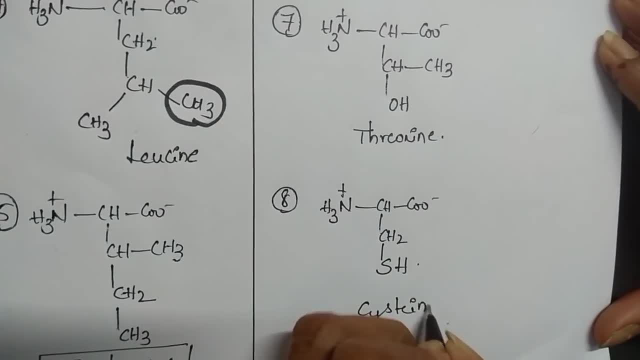 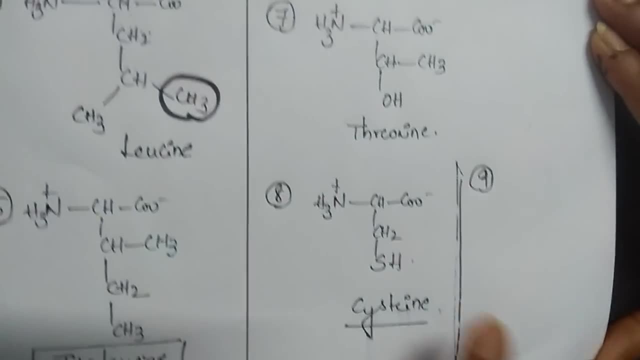 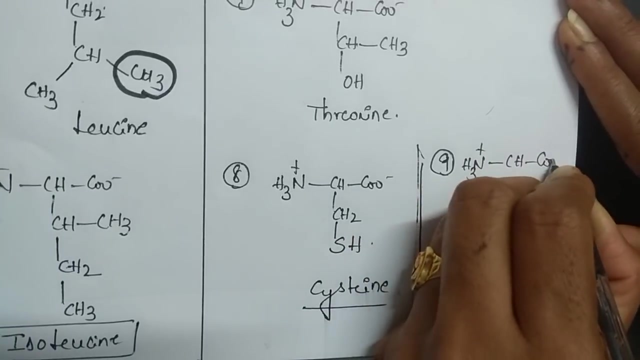 Okay, Its name is cysteine. What is its name? Cysteine? And here I am going to teach you one more structure. It is same like a cysteine. Little change I am doing: NH3 plus CHCO minus. This part is same. Only R group is changing. 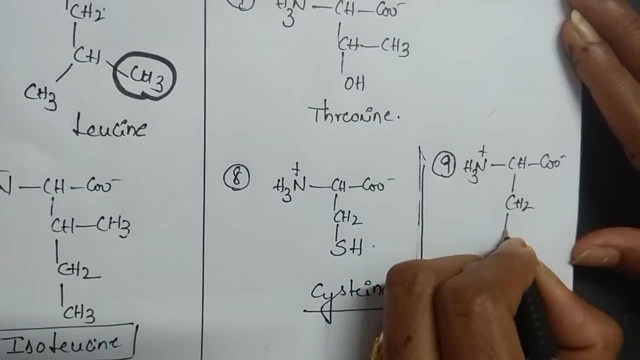 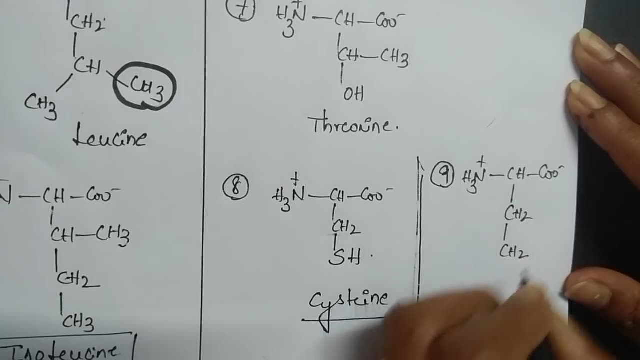 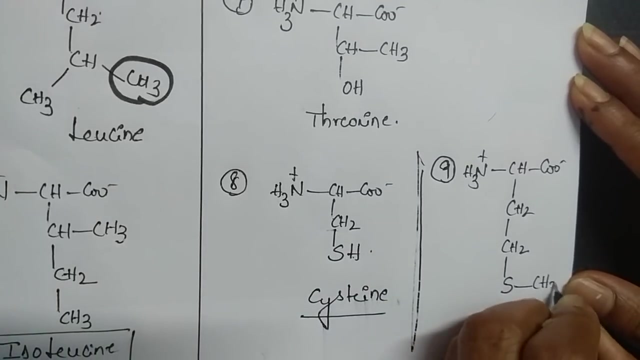 right. Even in R group this is same structure, But before this sulfur, here one CH2 group and here one CH2 group. So CH2, one group here and on sulfur extra CH2 group. I am keeping. So already one H is there CH2 and H is CH3.. So here one CH2, here one CH2 we are introducing. 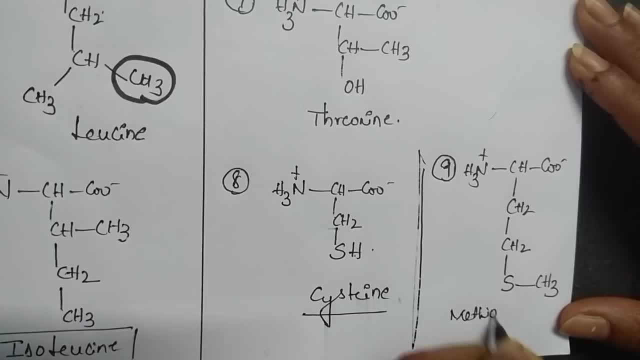 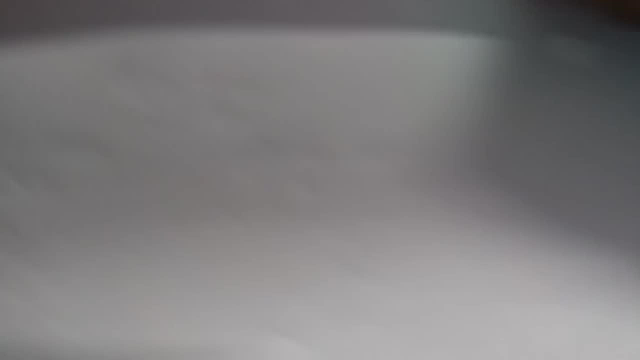 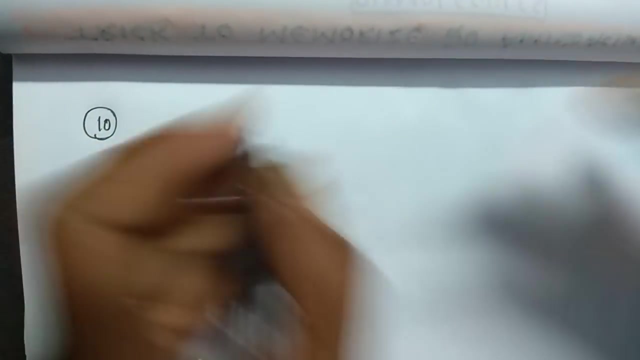 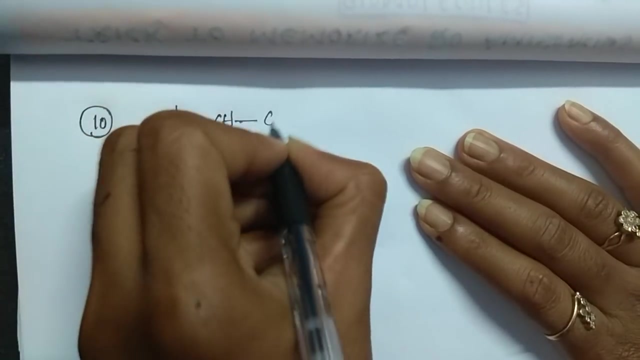 its name is methionine. What is the name of this amino acid, students? Methionine Clear. We completed 9 amino acid structures. Okay, Next 10th amino acid structure is- I am going to take same structure like alanine, Alanine. What is alanine structure? NH3 plus CH and CO minus. 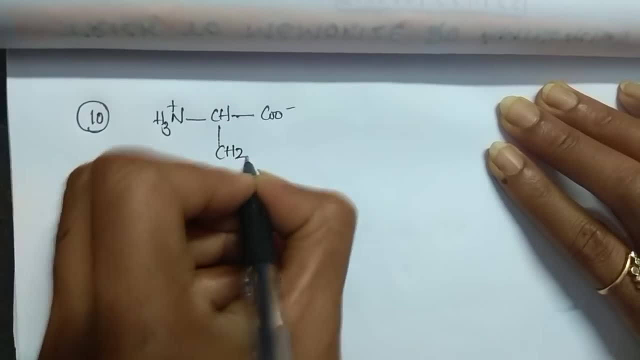 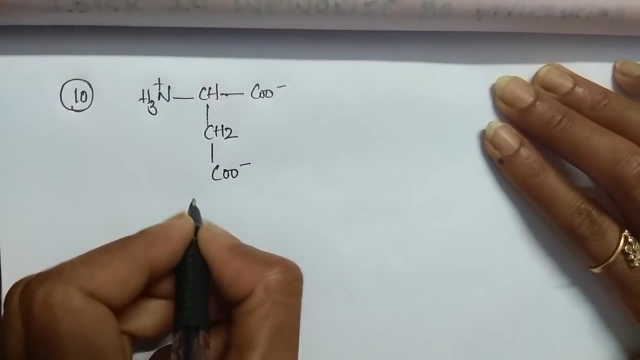 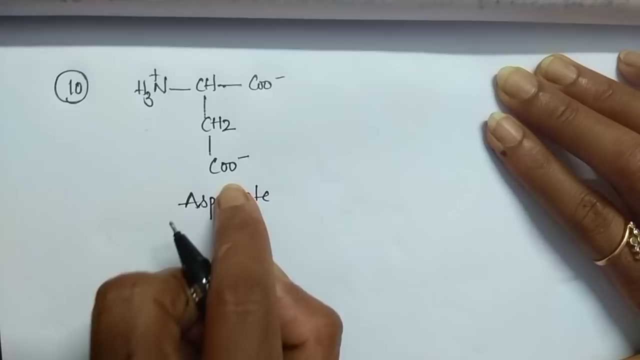 Here. CH3 is alanine, Right, So I am removing one hydrogen from it and I am going to put CO minus. Okay, Its name is aspartate. Aspartate- You can write here- NH2, COOH, COH, Normal form. 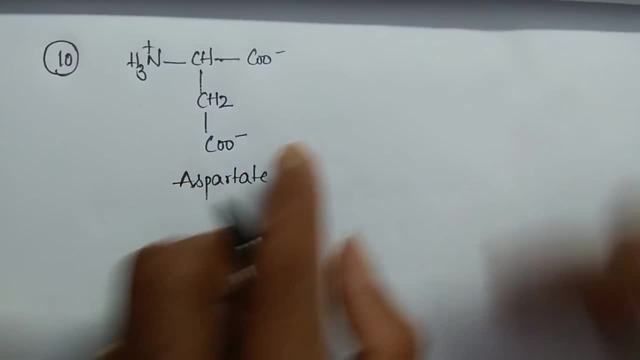 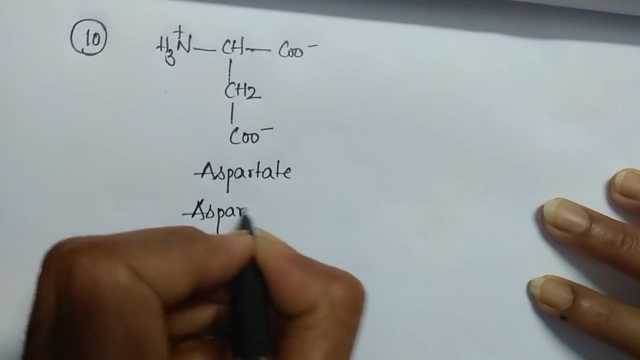 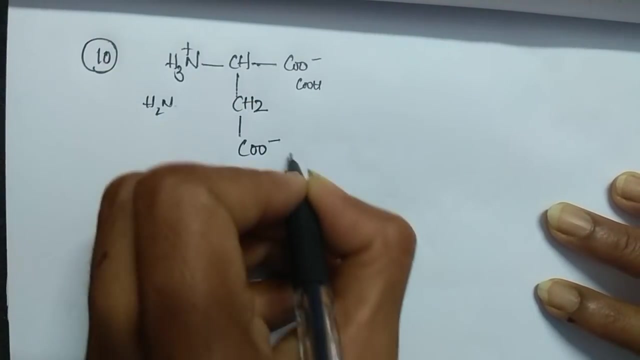 of amino acid. also, you can write without the ionic form. If you write here COH, COH, then it will become aspartic acid. What is its name? Aspartic acid, Aspartic acid- Okay, Here NH2 and here COOH, COH, It will become aspartate- Same structure. 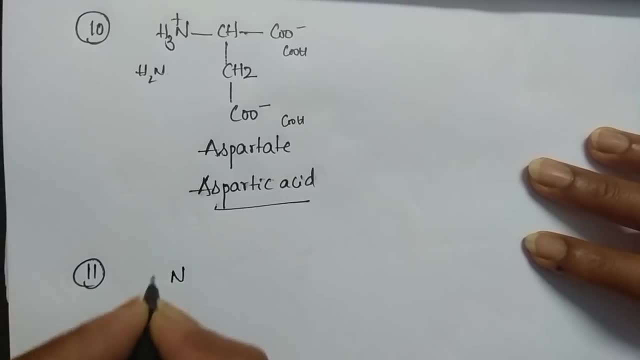 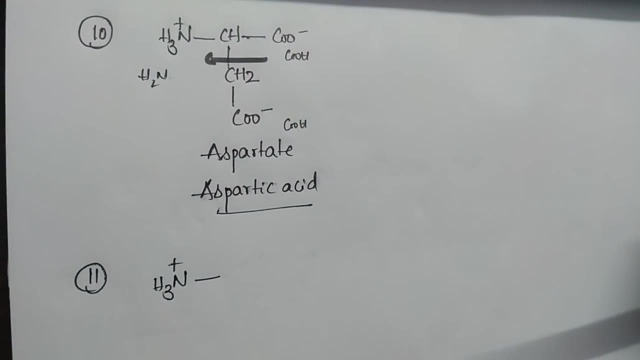 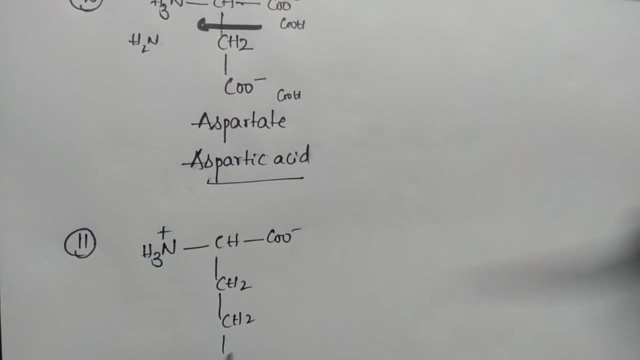 with this form And next structure is next structure is one more. a simple trick here is: keep one more CH2 extra, Then your structure becomes glutamic acid. What is its structure, But ionic form? I am writing here glutamate. 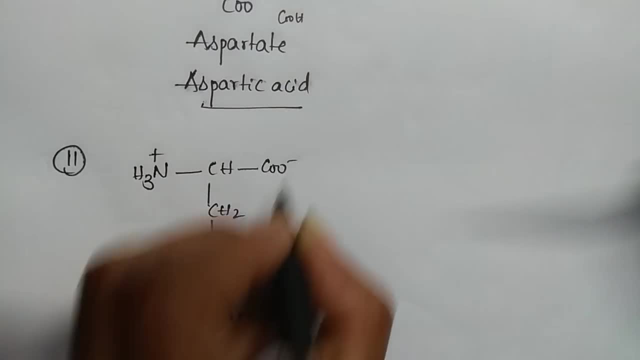 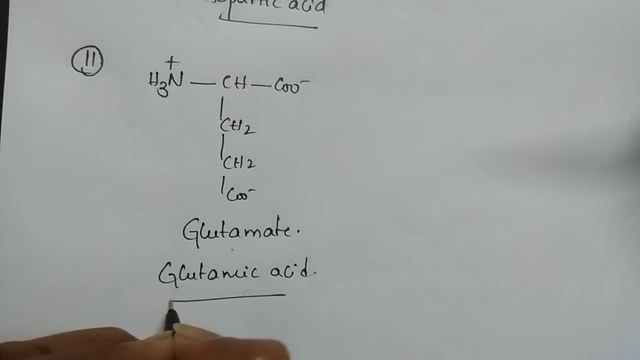 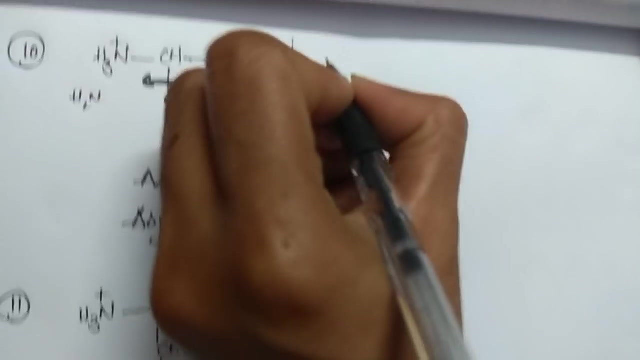 Or if you don't write ionic form, you put COH, COH and all. then it is glutamic acid, which you see in NCRT. Glutamic acid is the name you observe in NCRT. Okay, And we completed 11 structures. Now I am going to draw 12 structure. This is same like aspartic acid, But a small. 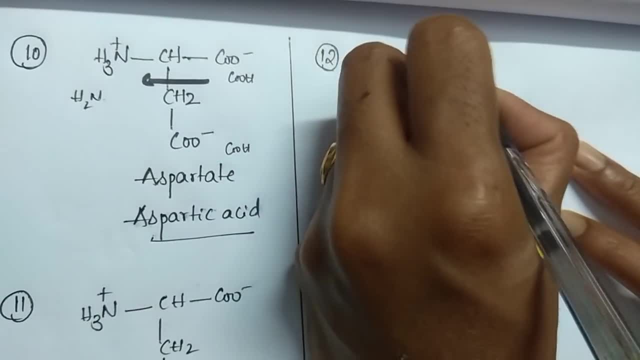 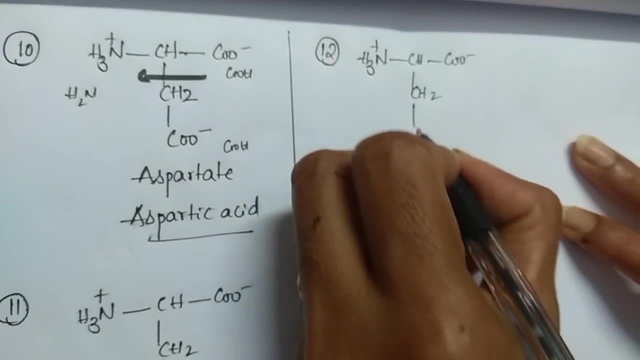 difference. See the small difference. What is the small difference? here I am going to write CH2.. Here COOH can be write CH2, COOH. That OH I am removing and I am keeping one, NH2.. Basic group: I am keeping. 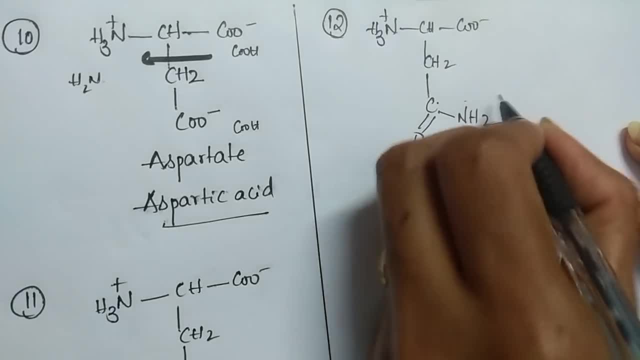 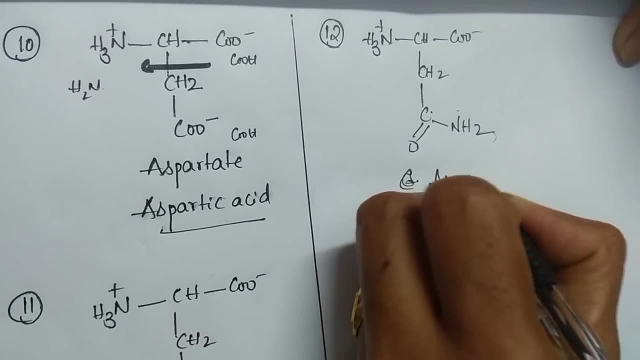 You can keep NH2 or you can keep NH3 plus also. Okay, Then its name is asparagine- Asparagine. What is its name? Asparagine? Next structure, 13th one, Same as that of glutamine 10 aspartic. 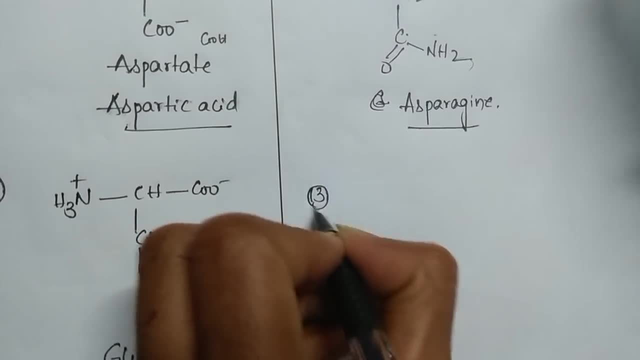 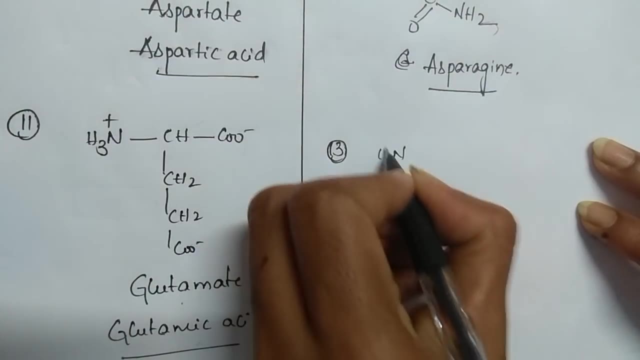 acid 4 chondroitol. Now I am keeping peroxin Right Here. CH is basic, No chondroitol Right And not strikeuras here. instead of COOH or COO minus I am going to place C double bond O NH2 amide group. I am 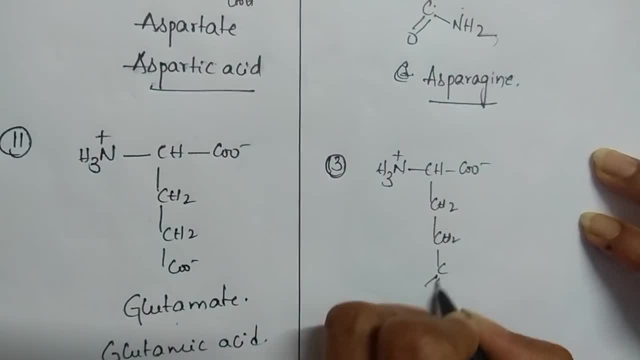 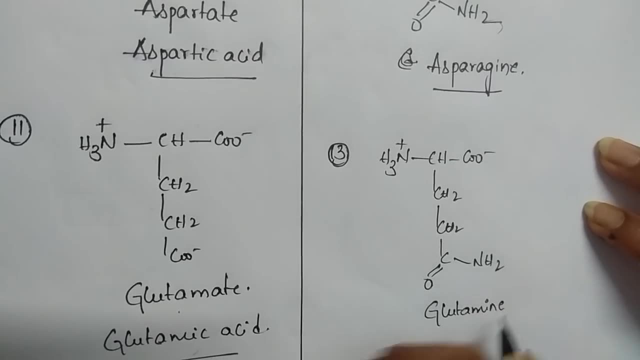 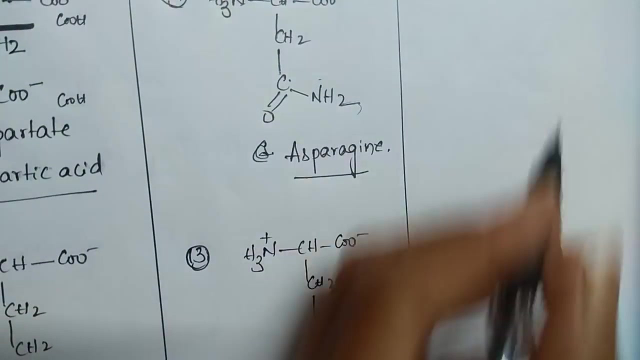 placing here. okay, then we get glutamine. what is the name of an amino acid? glutamine- amino acids- combines with each other, loss of water takes place and we get proteins. these are building blocks of proteins. okay, now I am going to draw 14th structure of amino acid. just write NH3 plus. 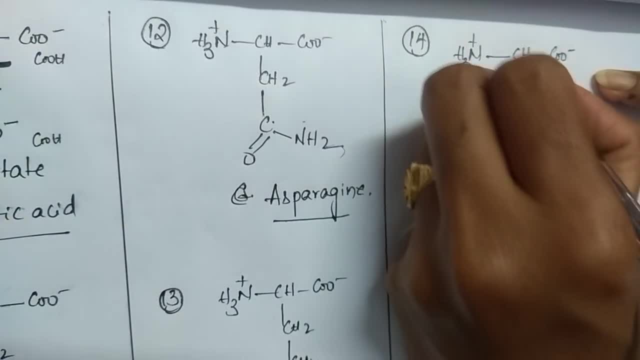 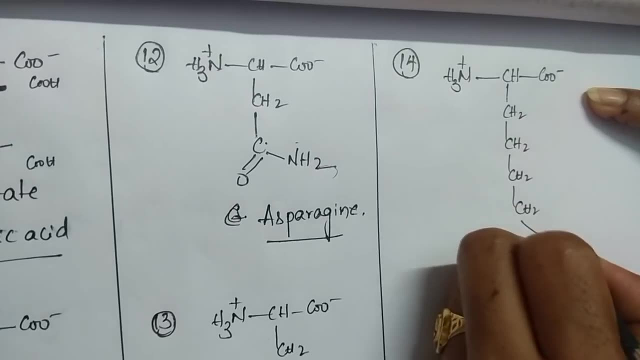 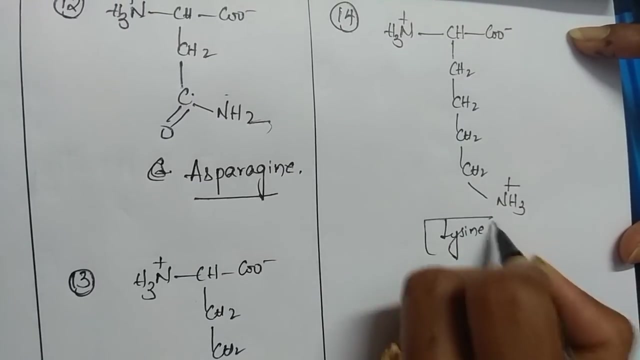 CHCOO minus. and here I am going to write 4 CH2 groups: see 4 CH2 groups. I am writing and I am placing 1 NH3 plus group here. its name is lysine. its name is lysine. 4 CH2 I kept and 1. 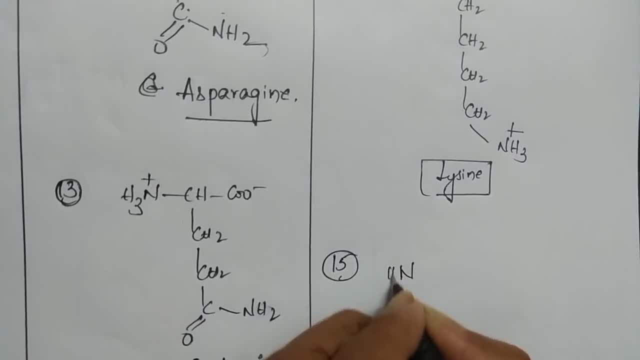 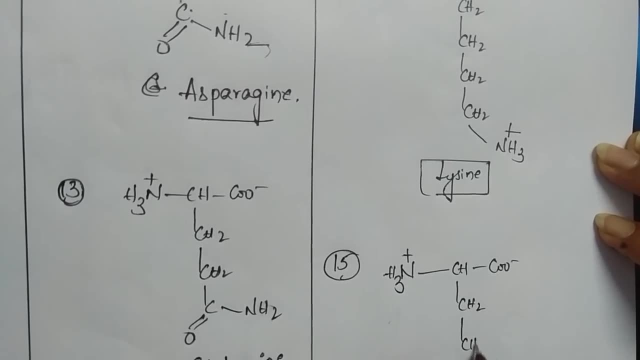 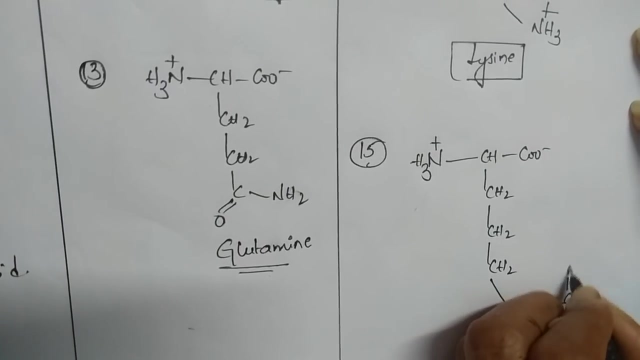 NH3 plus is Fe, presentation plus group. and next structure is: instead of 4 CH3s, I am going to place, just you know, just you know, 3 CH3 groups, CH2 groups, and here I will place 1, NH and C, double bond NH and here NH2. 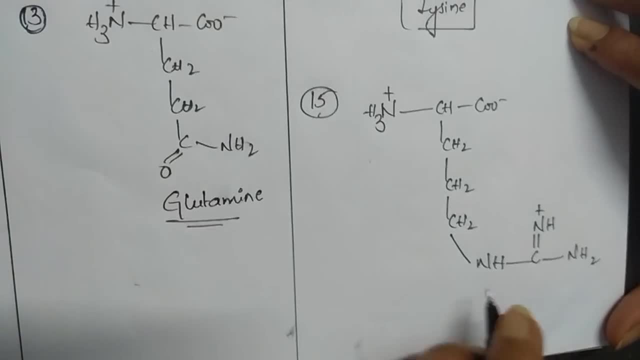 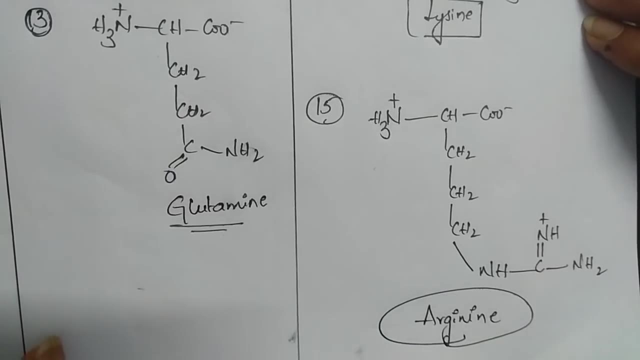 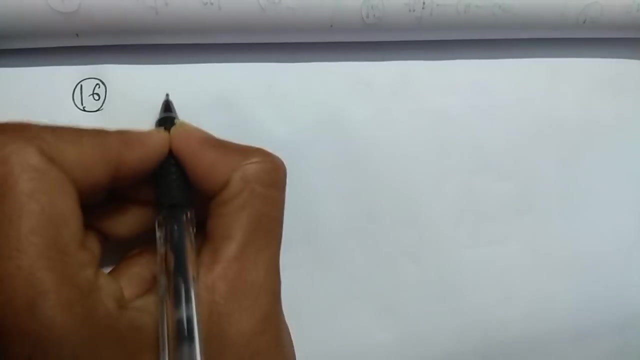 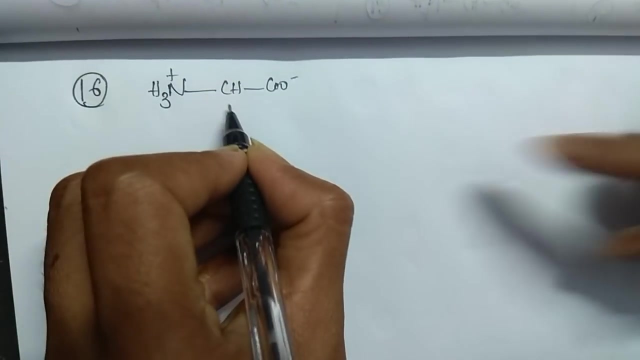 see, this is the structure. this is the structure of what? arginine? what is the name of this amino acid? arginine? clear, clear. and now I am going to draw the next structure. now I am going to draw 16th structure. take same alanine structure. okay, same alanine structure. here alanine means you. 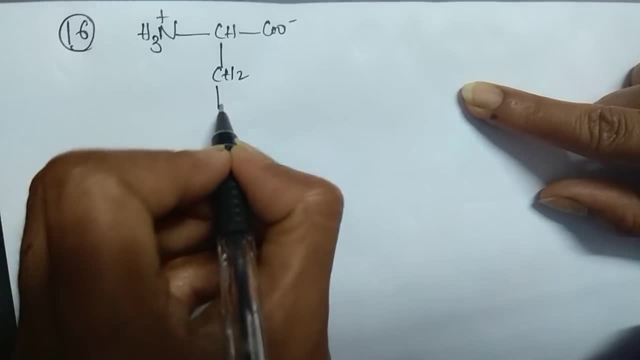 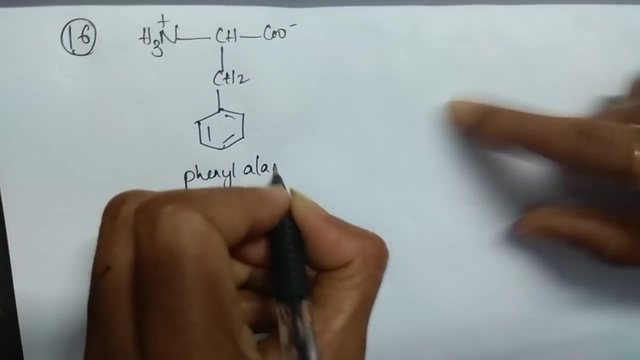 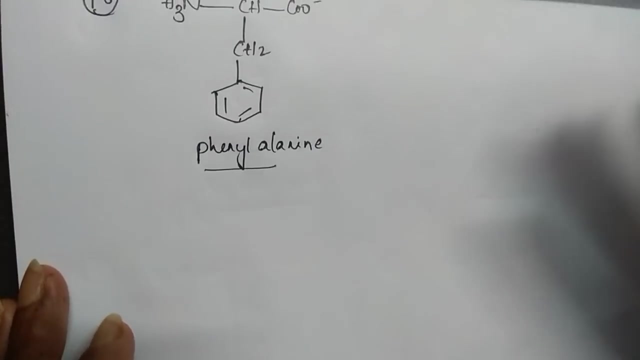 have to put CH3. I am going to remove 1 hydrogen, put and phenyl group. okay, this is called phenyl alanine. normally it is alanine. if you put only CH3, remove 1 hydrogen and keep a benzene ring, then it becomes phenyl alanine, right. next one is next. 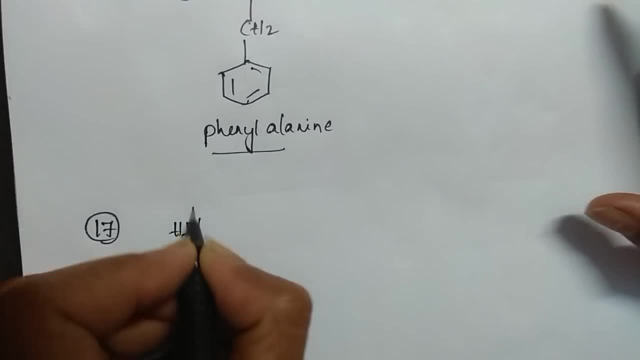 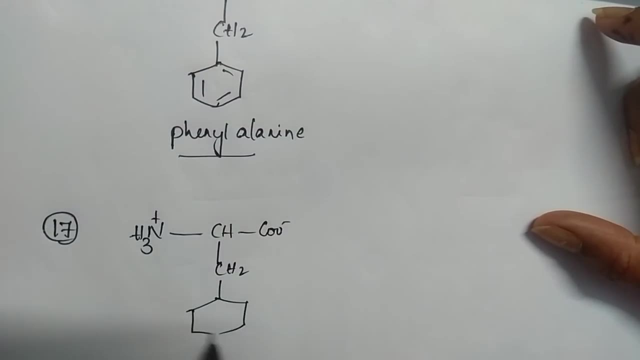 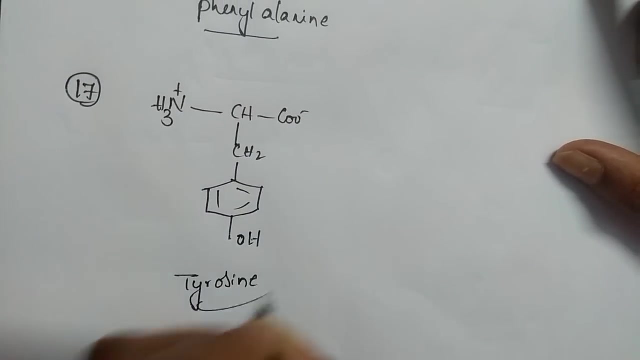 structure, same phenyl alanine structure you take, and at para position, at this position, see here at. at para position means this position put 1 OH group. this is called thyrosine. what is the name of this amino acid? thyrosine? we completed 17 structures. little slowly I am going to draw. 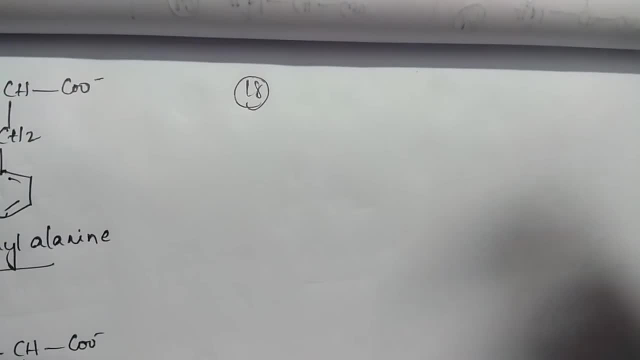 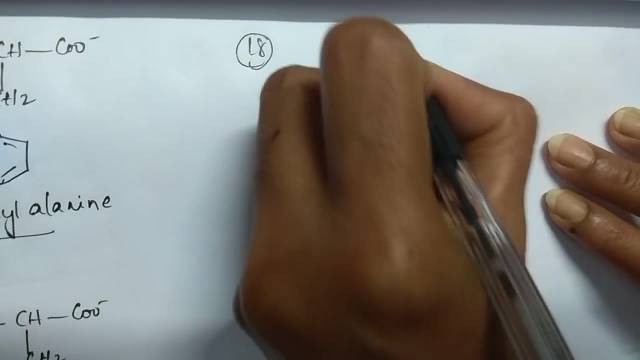 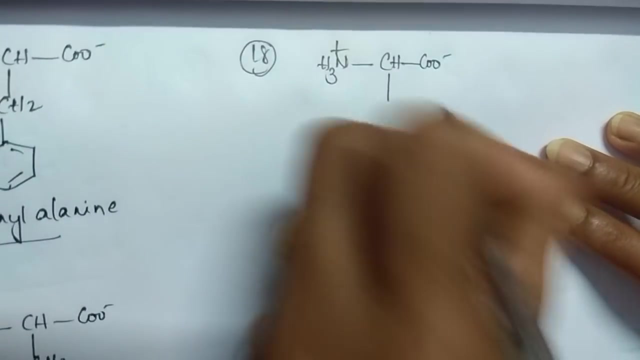 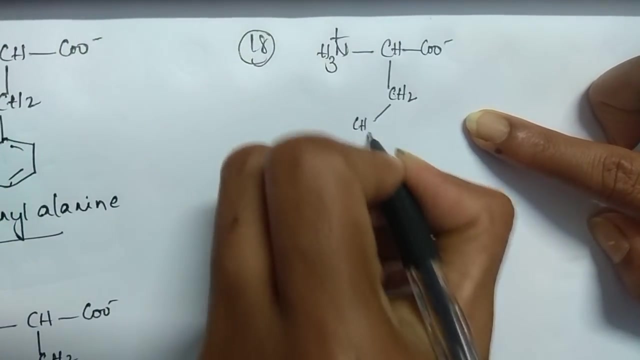 but you know, now I am going to teach you an amino acid. students feel difficulty of this amino acid concentrate. here I am going to give you super trick: CH, you know, COO minus, here NH3 plus correct, and here an alkyl group is there right? so what I am going to do is right here: CH2, CH2, CH2 and 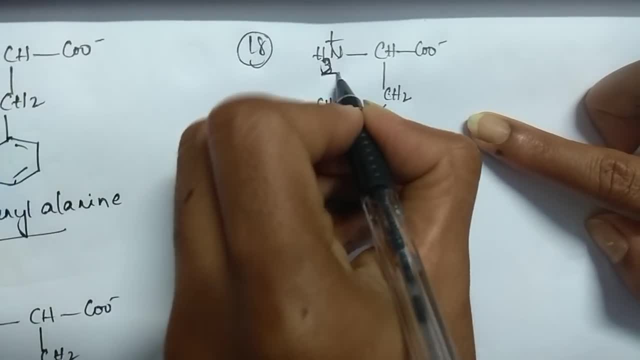 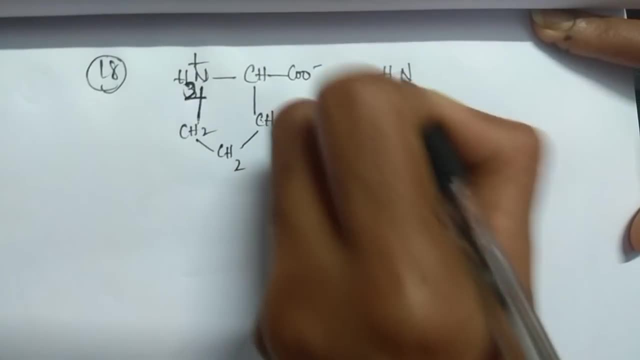 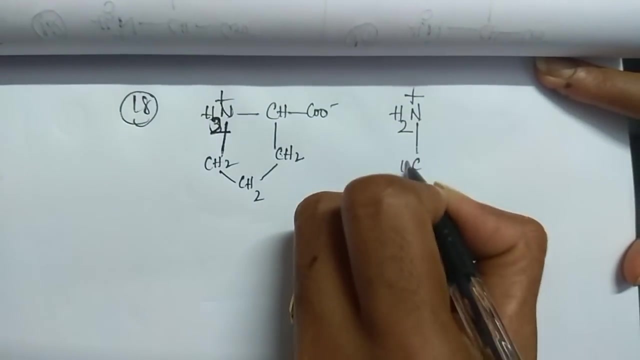 remove 1 hydrogen from this group. remove hydrogen from this group, then it becomes NH2 and connect these two again. I am drawing see NH3 plus. I am removing 1 hydrogen, so that what I am going to do is I am going to put a bond, a connection, a. 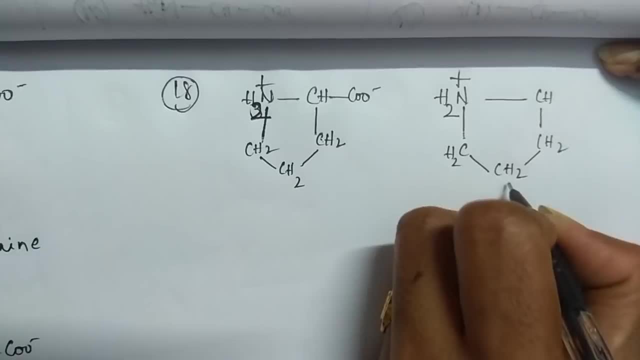 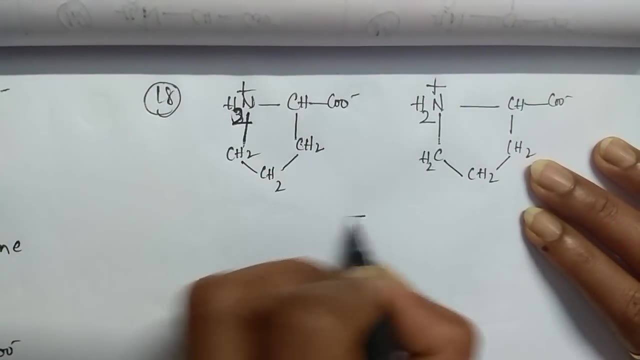 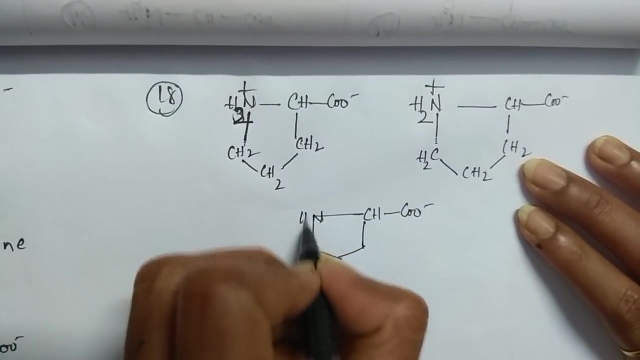 connection between these three CH2, CH2, CH2- I am giving one connection here, so I removed one bond here, so I removed one hydrogen, same structure. you can see like this enough and see everything is perfect. look here, I am drawing like this. you can see that this is a tweet. 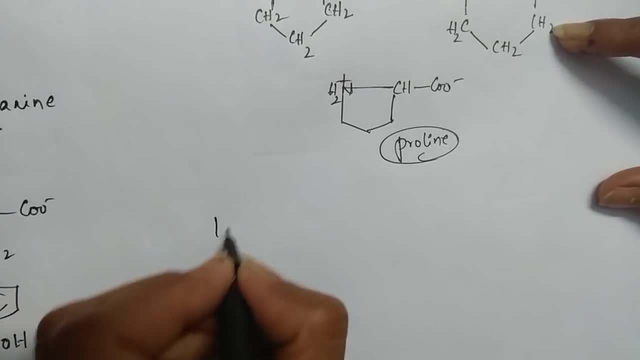 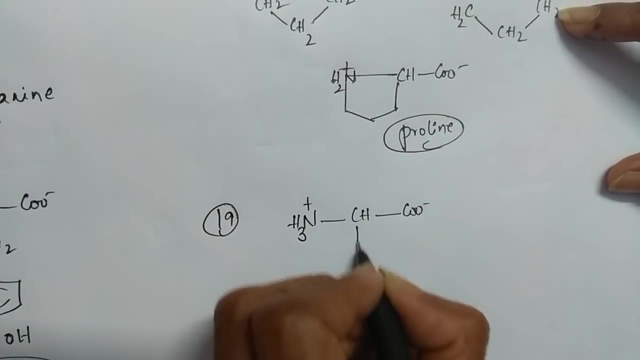 write this само B, NH2 plus, and it's the name of an amino acid. students rolling next in 19 structure. observe carefully, observe carefully. histidine is a structure you feel difficulty to draw, but see how easily you can draw. just to draw a five membered ring. okay, five membered ring. once you draw a five membered ring or a 5 membered ring, you can draw a 5 membered ring. it's really easy. okay, just to draw a 5 membered ring. and when you draw an five membered ring, you can see that it's easy, right. 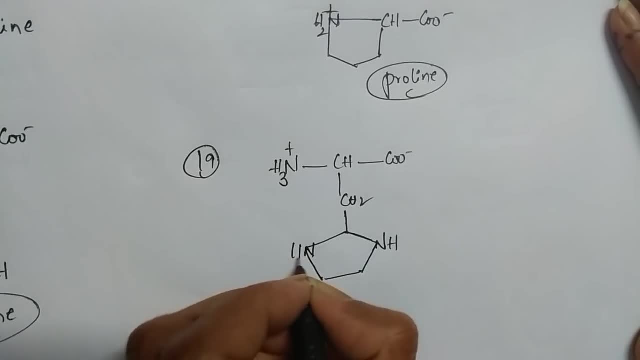 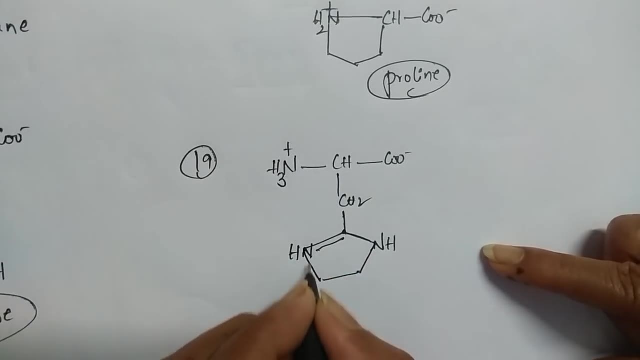 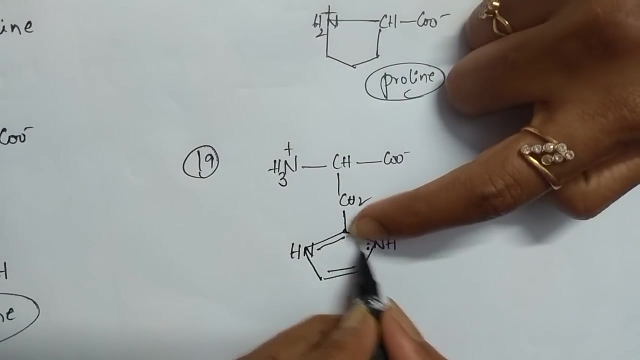 ring like this: put one nh here, one nh here, okay and just this is the bond position to this ring. and put one double bond here, leave one bond again. put one double bond and again here, lone pair. if you start bonding here, put one bond here. here one more bond here, lone pair, your wish, but here. 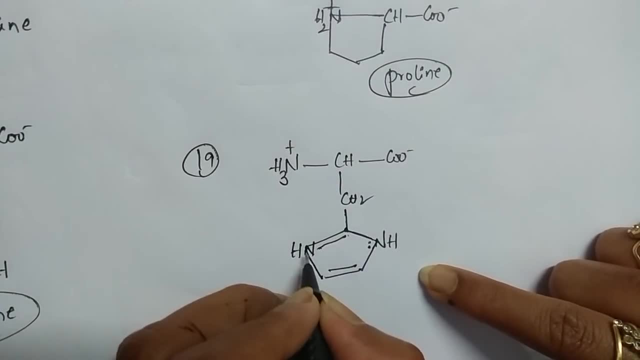 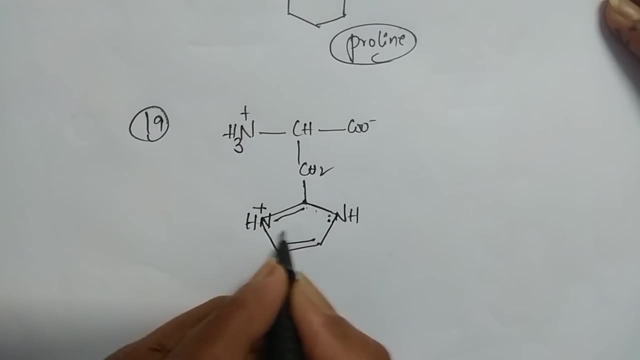 you have to. if you observe one, two, three, four bonds is there, so you have to put a positive charge on this. this here, this lone pair, is in conjugation with this is an aromatic ring. okay, this is called histidine. what is the name of an amine acid, histidine? now i am going to teach. 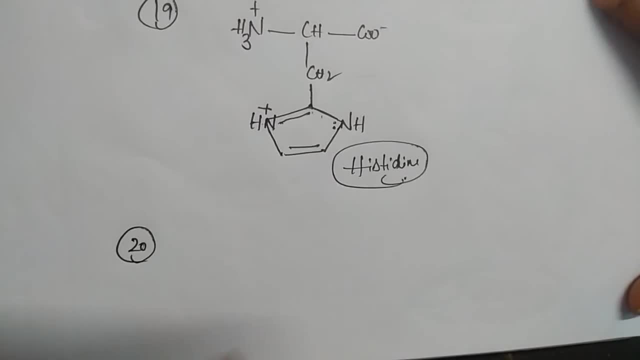 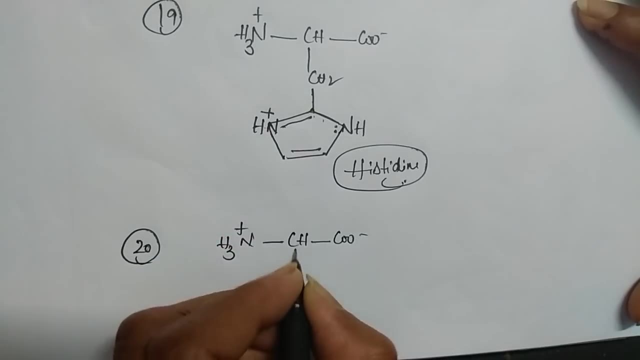 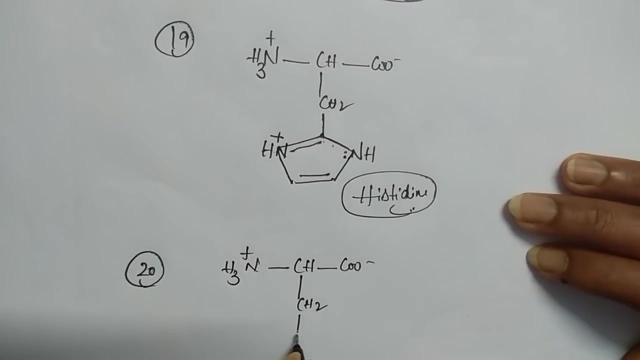 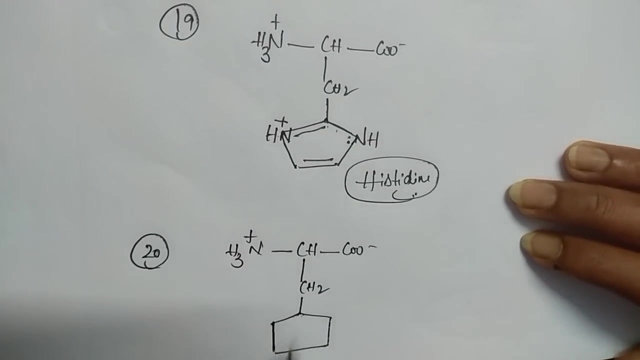 on 20th amine acid. this is the last amine acid. here i am going to write co minus and nh3 plus, here and here ch2. here also draw a five membrane ring. but the six, six, six, six simple trick here is you have to put a bond straight here your wish how you draw the remaining. 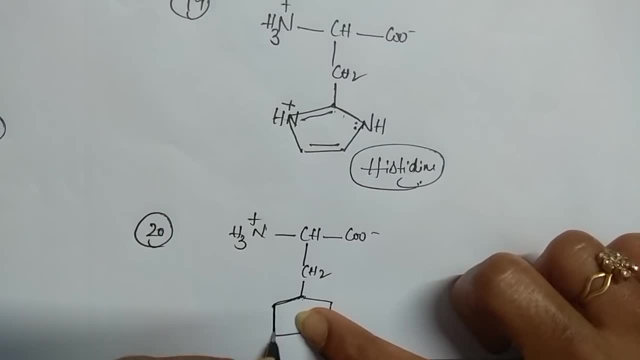 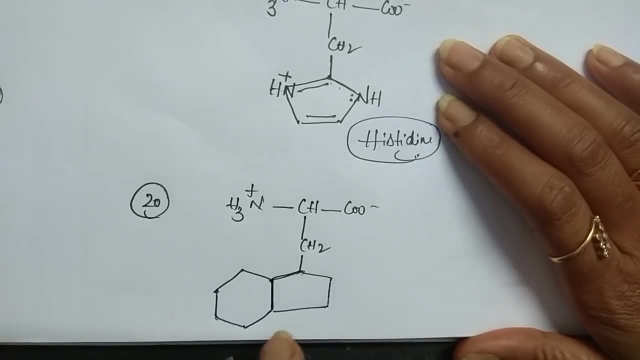 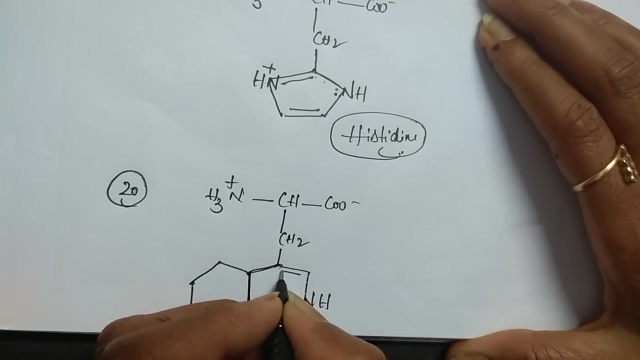 part, but main part is one bond like this. one bond. it should be straight, otherwise your structure becomes a wrong. then you put one benzene ring. okay, now he from here. you start giving here nh. you write: leave one bond, put a double bond. leave one bond, put a double bond. leave one bond, put one. 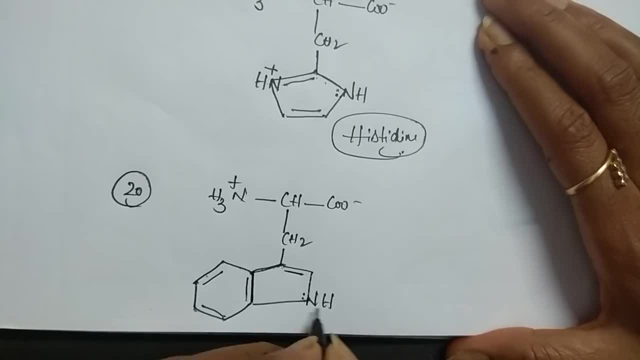 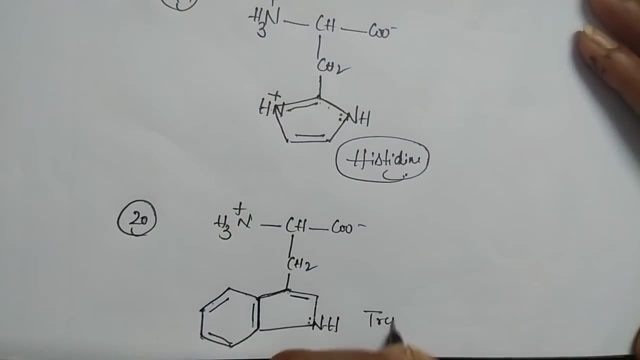 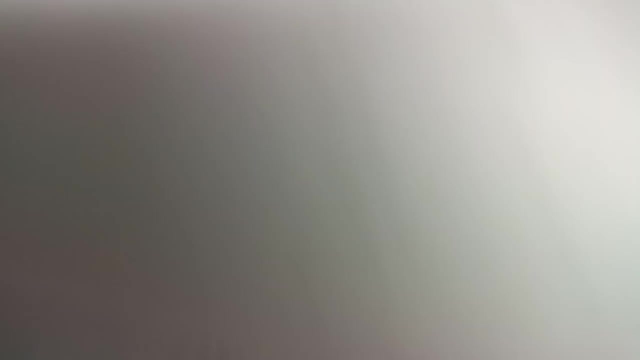 double bond. leave one bond, put double bond, that's it. if you observe here, nitrogen is having three bonds, right, so as usual, it lone pair will be. its name is tryptophan. tryptophan- got the clarity, got the clarity. this is about 20 amino acid structures and 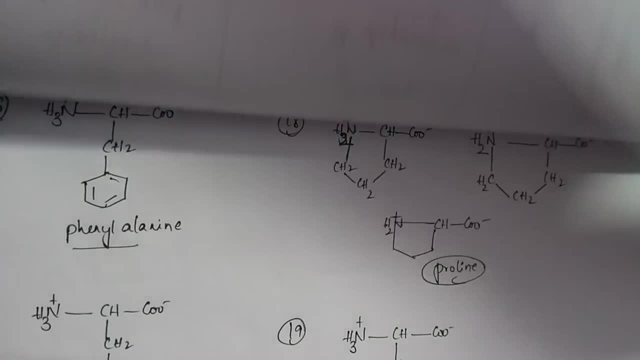 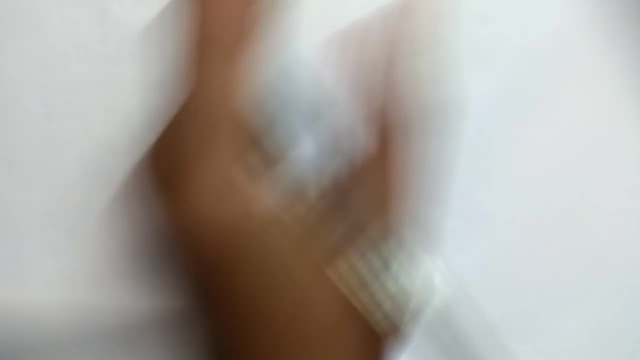 now i am going to give you a trick for trick for av hill mptt. as i told you, i am going to teach you that a av hill mptt. but this video is almost 14 minutes cross. so next video i am going to give you. 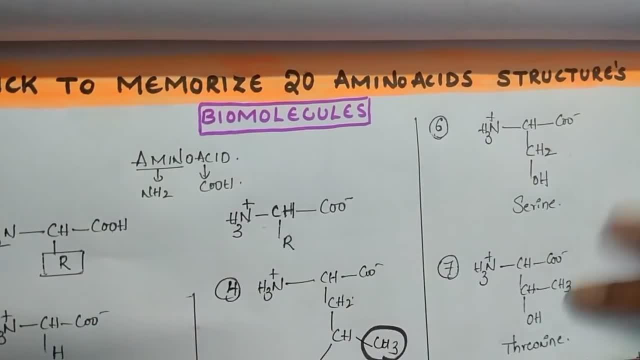 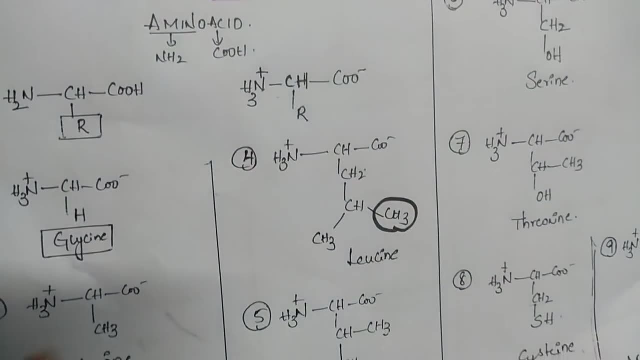 the trick. what is that? av hill, mptt, practice this. all. draw the structures and practice one time. definitely it becomes very easy for you. amino acids: my name is komali. i am your chemistry mentor. thank you so much for watching this video.